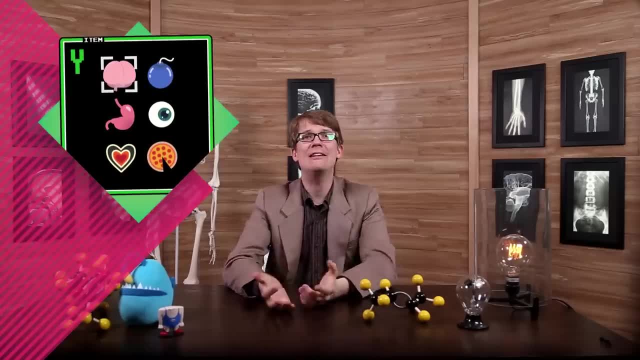 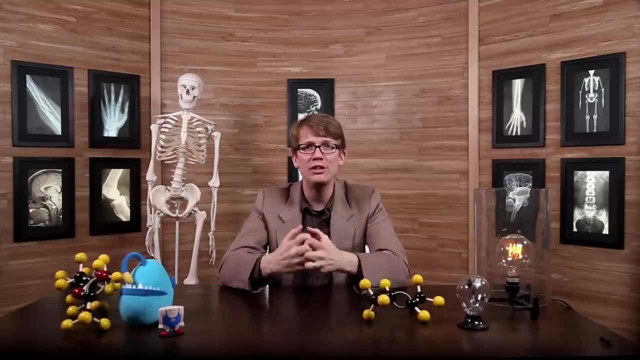 lots of Latin gobs of Greek. But this course isn't just going to be an inventory of your individual parts or a diagram of how a slice of pizza gives you energy, Because these disciplines are really about why you're alive right now and how you came to be alive, how disease 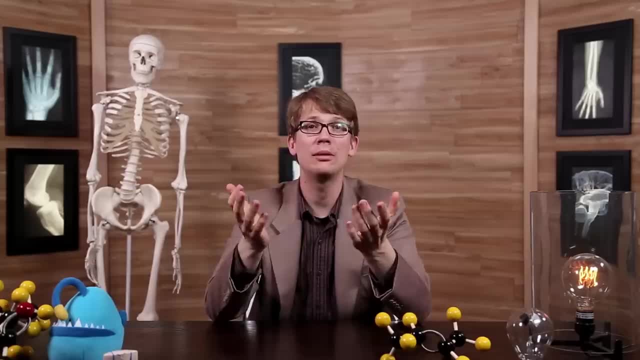 harms you and how your body recovers- And it's a lot of science, but it's a lot of science too- and how your body recovers from illness and injury. It's about the big picture stuff that we either spend most of our time thinking about or 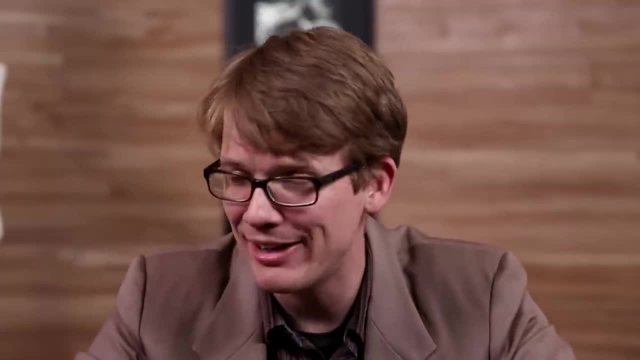 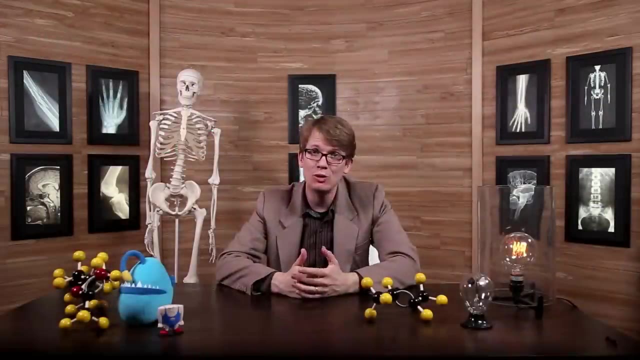 try not to think about Death and sex and eating and sleeping and even the act of thinking itself, All processes that we can understand through anatomy and physiology. If you pay attention and if I do my job well enough, you'll come out of this course with 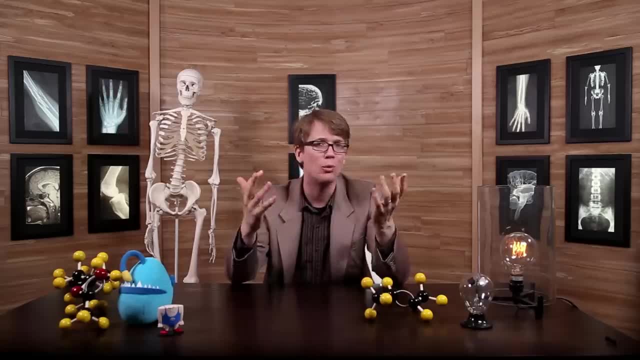 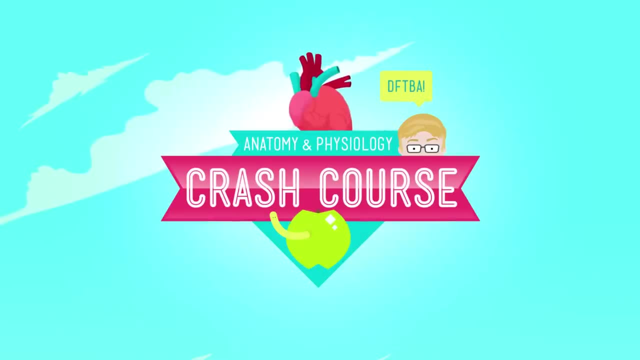 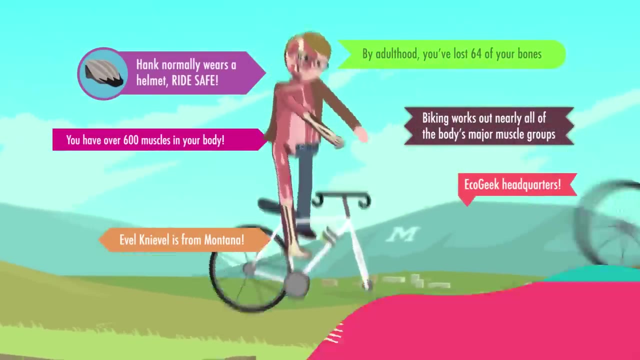 a richer, more complete understanding, not only of how your body works- everything from handshakes to heart attacks- but I think you'll also start to see that you really are more than just the sum of your parts. We've come to understand the living body by studying a lot of dead ones And for a 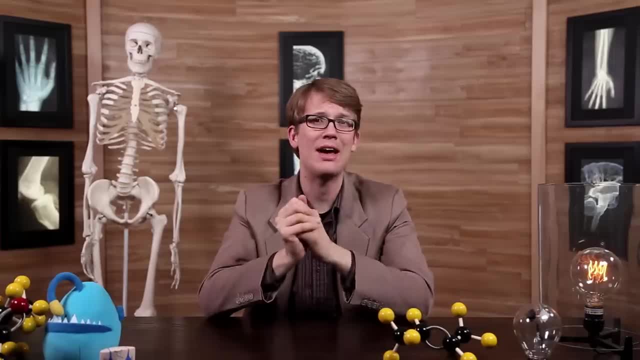 long time we did this mostly in secret. For centuries, the dissection of human bodies was very taboo in many societies and, as a result, the study of anatomy has followed a long and slow, and often creepy, road. The second century Greek physician, Galen, gleaned what he could about the human form by performing 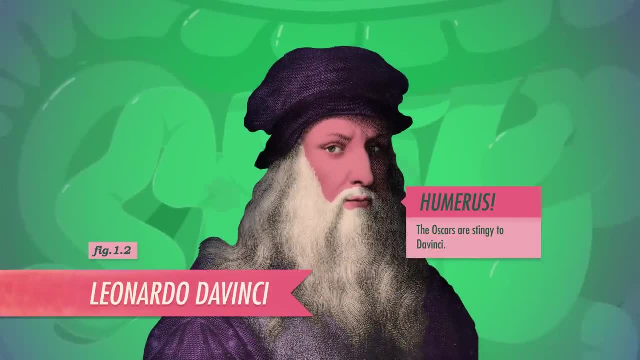 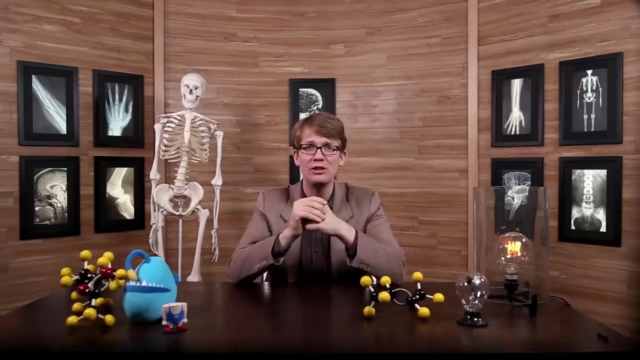 vivisections on pigs. Da Vinci poked around in dead bodies while sketching his beautifully detailed anatomical drawings until the Pope made him stop. It wasn't until the 17th and 18th centuries that certified anatomists were allowed to perform. 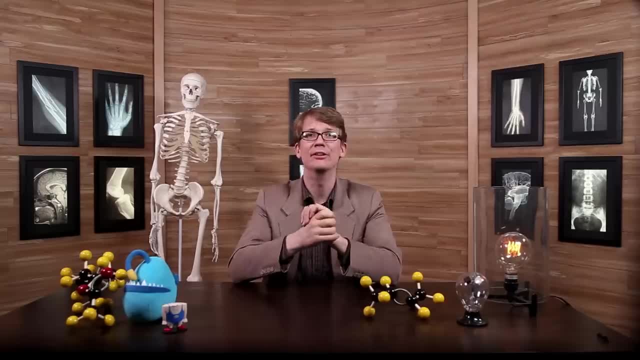 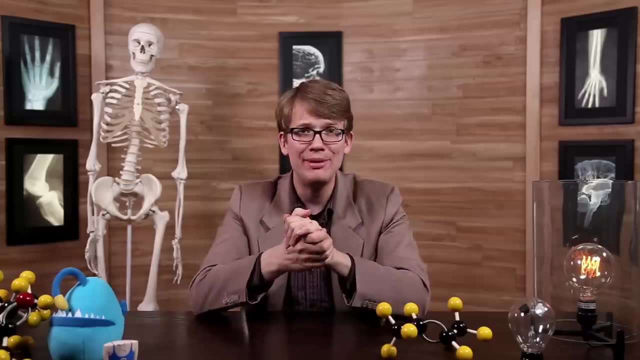 tightly regulated human dissections, And they were so popular that they were often public events with admission fees, attended by the likes of Michelangelo and Rembrandt. The study of human anatomy became such a craze in Europe that grave robbing became a lucrative if. 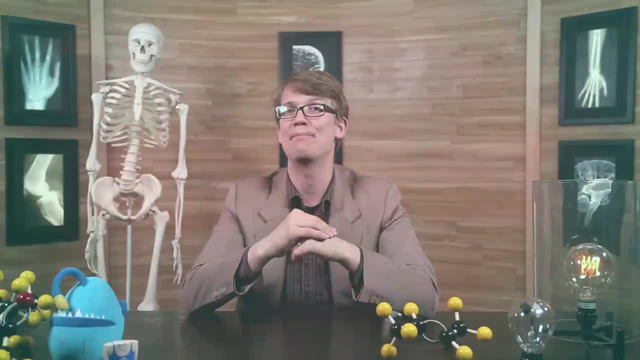 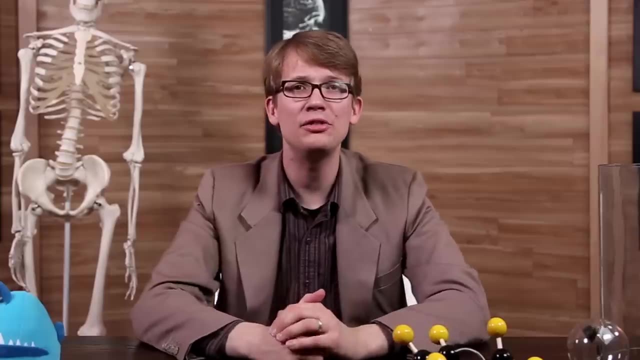 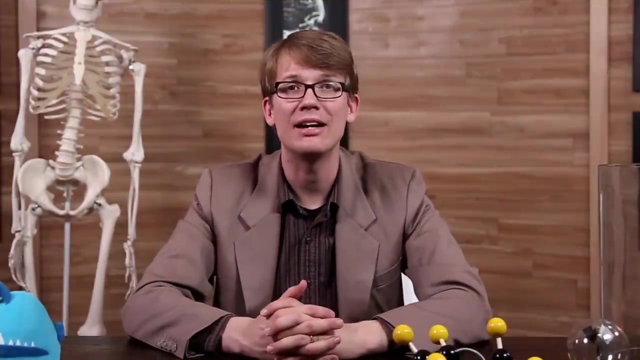 not legal occupation. It was in 1832 when Britain passed the Anatomy Act, which provided students with plentiful corpses in the form of executed murderers. Today, students of anatomy and physiology still use educational cadavers to learn in person and hands-on what's inside a human body by dissecting them. 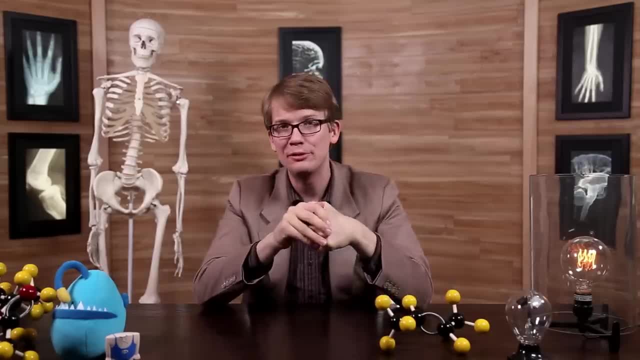 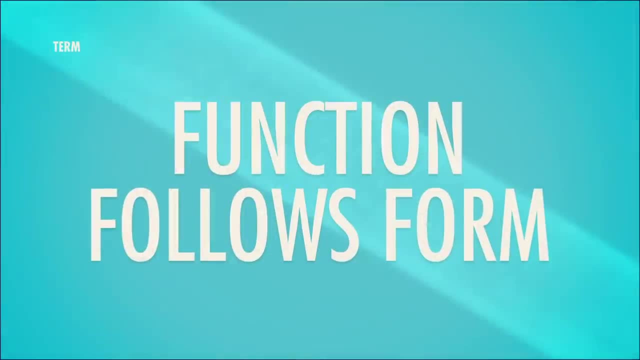 And it's totally legal. The cadavers are volunteers, which is what people mean when they say that they're donating their body to science. So what have all these dead bodies shown us? Well, one big idea that we see over and over again is that the function of a cell or an 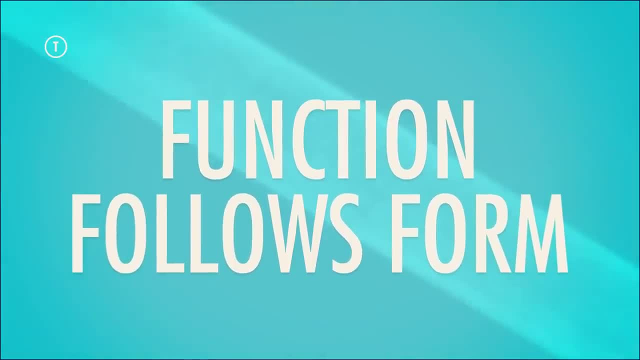 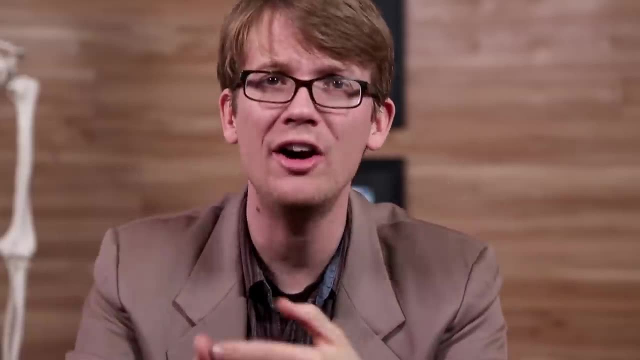 organ or a whole organism always reflects the body. So what does that mean? It reflects its form. Blood flows in one direction through your heart simply because its valves prevent it from flowing backward. In the same way, your bones are strong and hard, and this allows them to protect and. 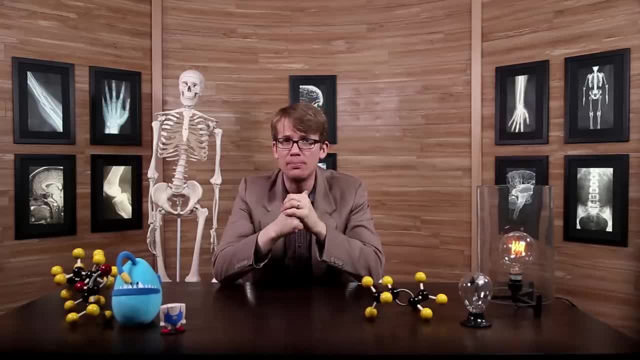 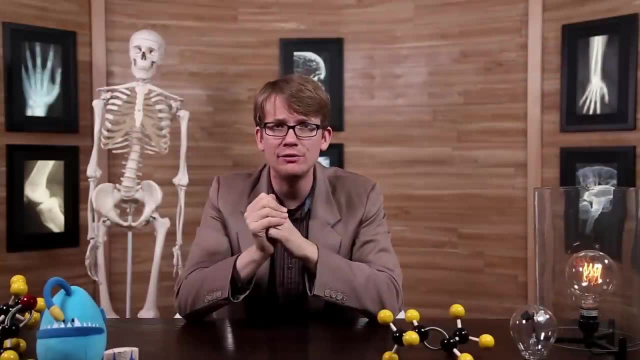 support all your soft parts. The basic idea that what a structure can do depends on its specific form is called the complementarity of structure and function, And it holds true through every level of your body's organization, from cell to tissue to system. And it all begins with the smallest of the small atoms. 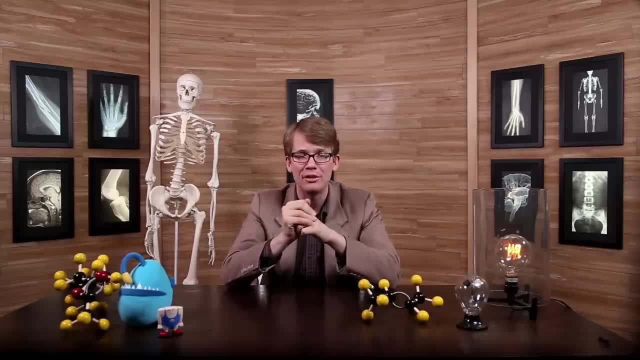 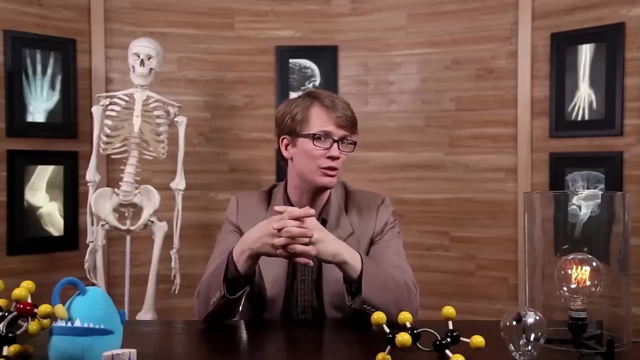 Just like the chair you're sitting on, you are just a conglomeration of atoms, About seven octillion of them to be precise. Fortunately for both of us here, we've covered the basics of chemistry that every incoming physiology student needs to know in Crash Course Chemistry. 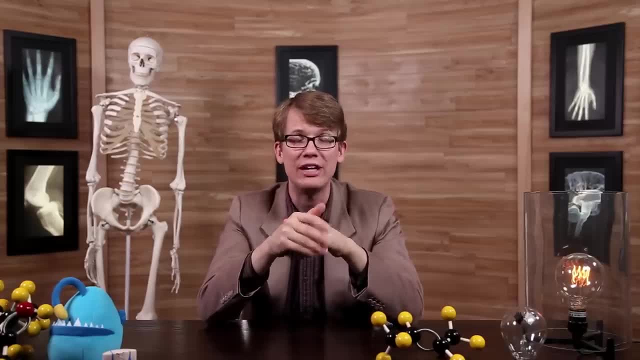 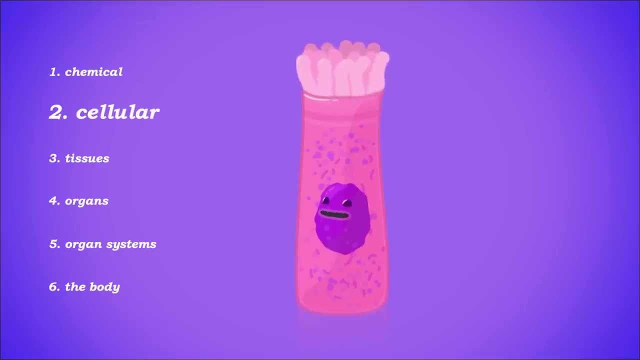 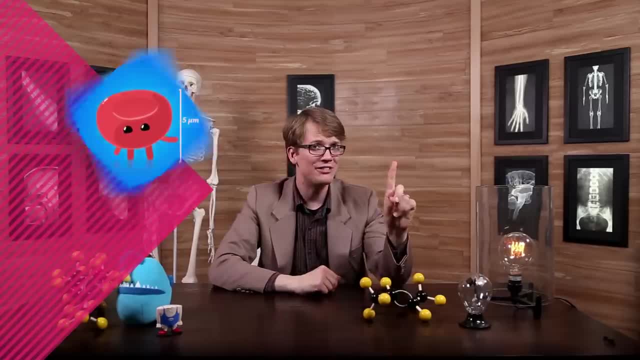 The red blood cells are the cells that make up the blood. The red blood cells are the cells that make up the blood. The red blood cell, which measures about 5 micrometers across. Now contrast that with the single motor neuron that runs the length of your entire leg from. 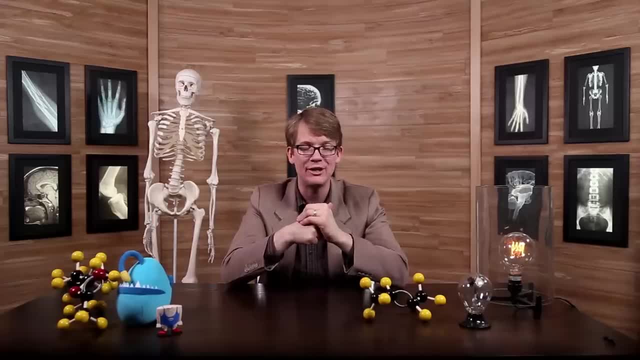 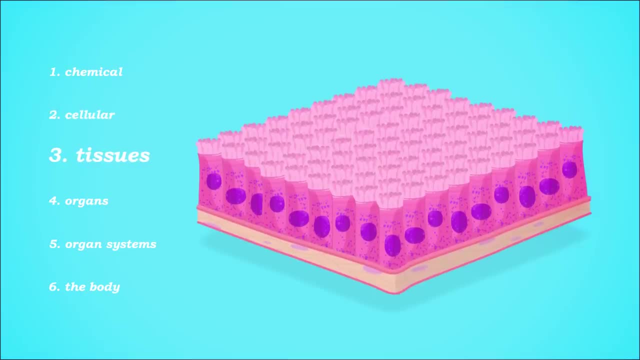 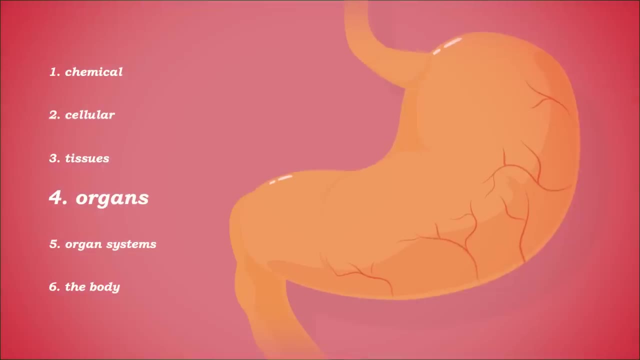 your big toe to the bottom of your spine, about a meter from end to end. Typically, cells group with similar cells to form the next level of organization- Tissues like muscles, membranes and cavity linings, nervous and connective tissues. When two or more tissue types combine, they form organs. 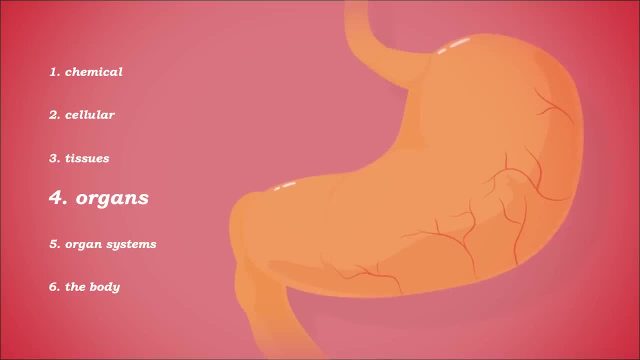 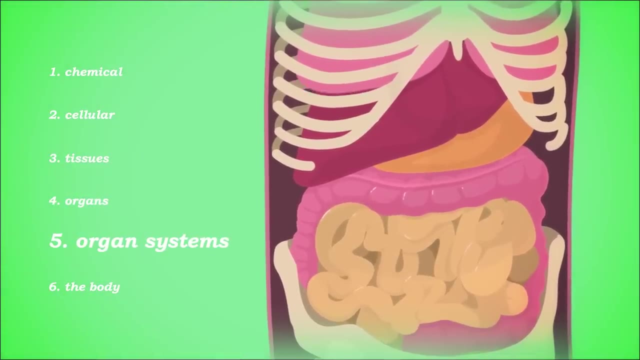 The heart, liver, lungs, skin and et cetera that perform specific functions to keep the, to keep the body running, Organs work together and combine to get things done, forming organ systems. It's how, like the liver and stomach and intestines of your digestive system, 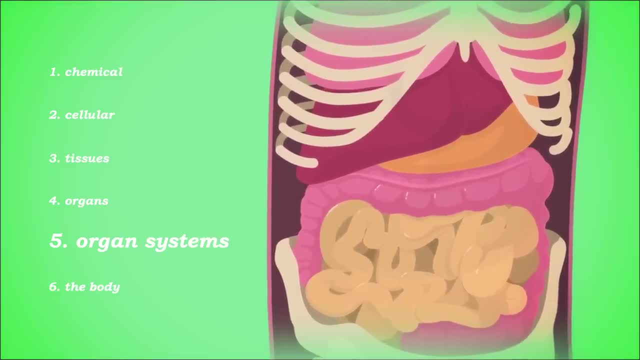 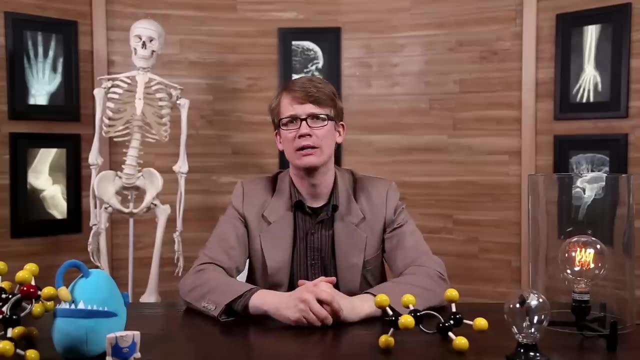 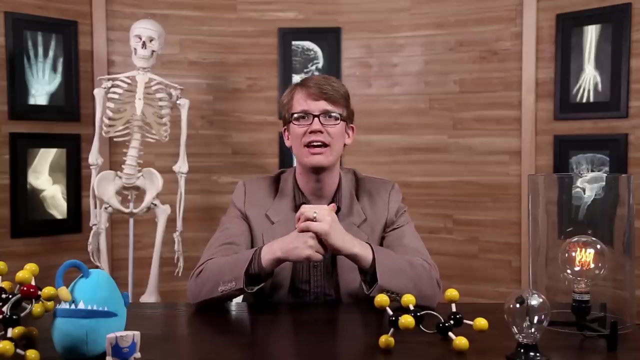 all unite to take that burrito from plate to pooper And finally, all those previous levels combine to form the highest level of organization: the body itself. Me and you and your dog, we're all glorious, complete organisms made from the precise organization of trillions of cells in nearly constant activity. 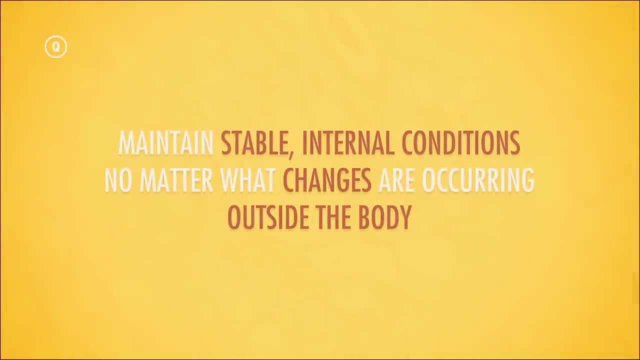 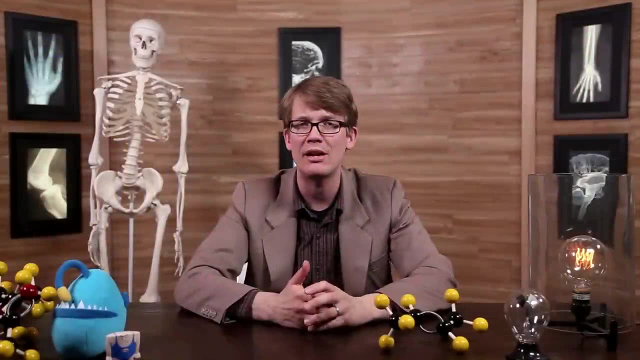 This ability of all living systems to maintain stable internal conditions no matter what changes are occurring outside the body is called homeostasis, and it's another major unifying theme in anatomy and physiology. Your survival is all about maintaining balance of both materials and energy. 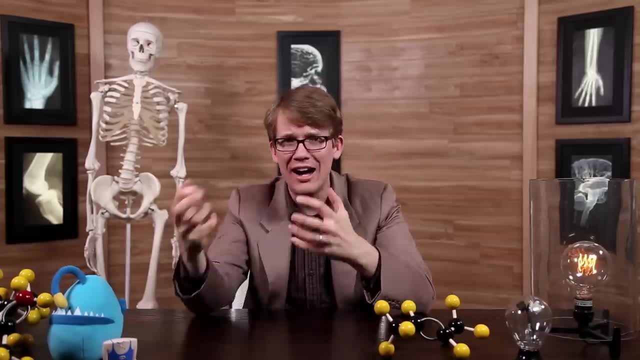 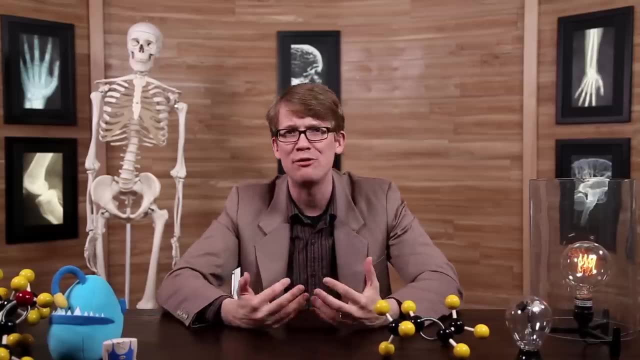 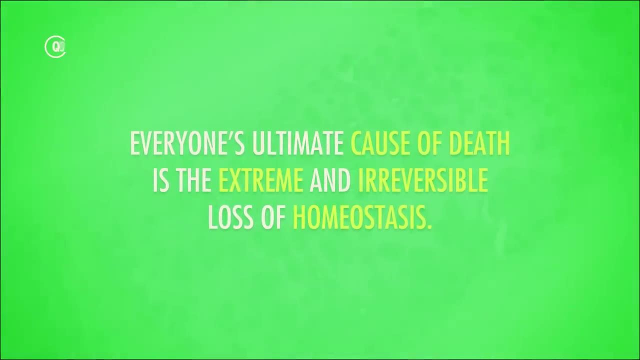 You need the right amount of blood water, nutrients and oxygen to create and disperse energy, as well as the perfect body temperature, the right blood pressure, the efficient movement of waste through your body. All that needs to stay balanced And by your survival depending on it. I mean that everyone's ultimate cause of death. 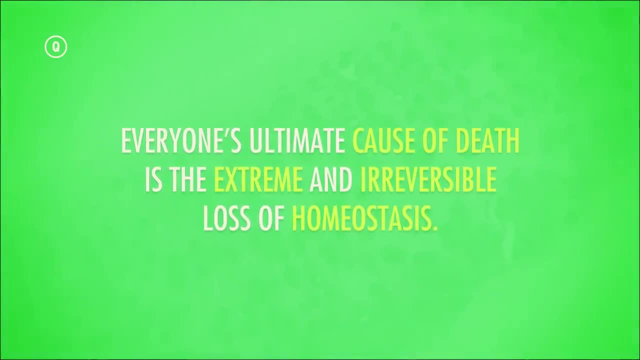 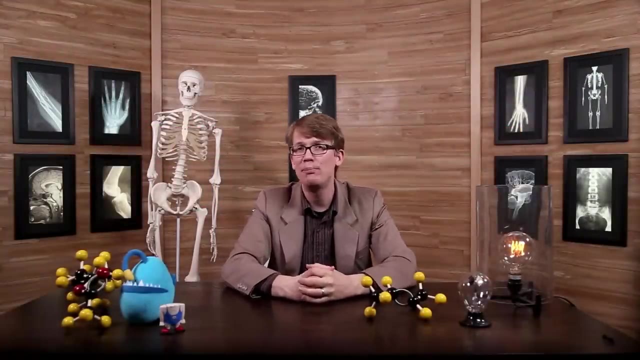 is the extreme and irreversible loss of homeostasis. Organ failure, hypothermia, suffocation, starvation, dehydration- they all lead to the same end: by throwing off your internal balances that allow your body to keep processing energy. Take an extreme and sudden case. Your arm pops off. If nothing is done quickly to treat such a severe wound, you would bleed to death. right, But what does that really mean? What's gonna happen? How do I die? That arterial wound, if left untreated, will cause a drastic drop in blood pressure. that 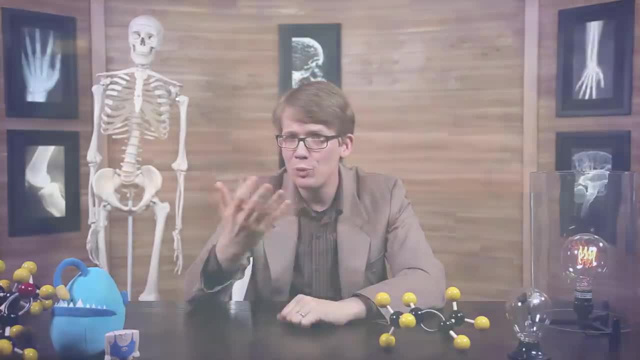 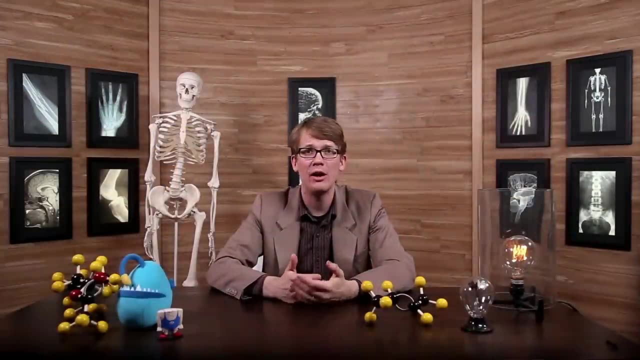 in turn will prevent the delivery of oxygen throughout the body. So the real result of such an injury, the actual cause of death, is the loss of homeostasis. I mean you can live a full and healthy life without an arm, but you can't live without 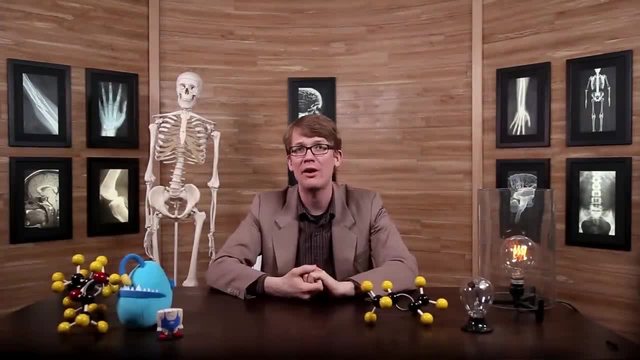 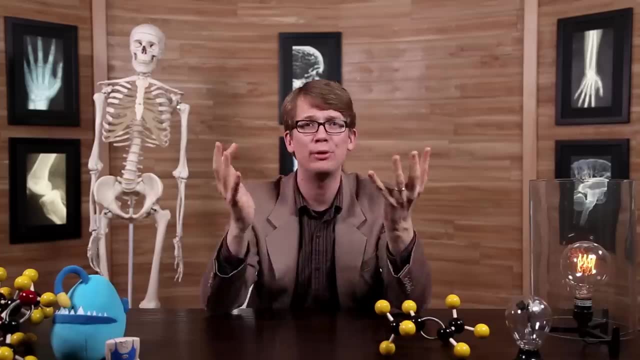 blood pressure, Because without blood, your cells don't get oxygen and without oxygen they can't process energy and you die. With so many connected parts needed to make your life possible, you can see how we need a hyper-precise language to identify the parts of your body that you need to process energy. 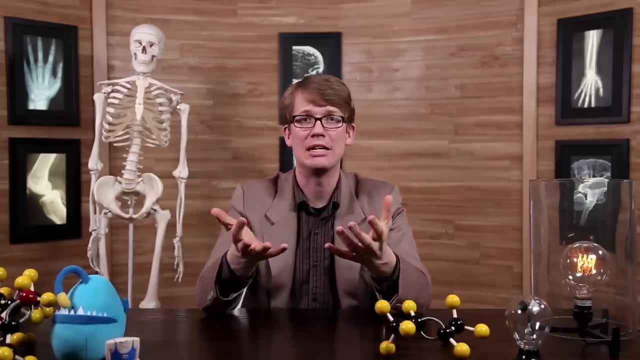 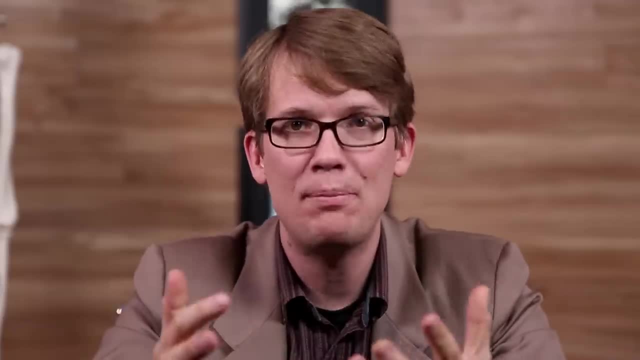 And that's what we're gonna do. We're gonna cut up parts of your body and communicate what's happening to them. A doctor isn't gonna recommend a patient for surgery by telling the surgeon that the patient has an achy belly. They're gonna need to give a detailed description. 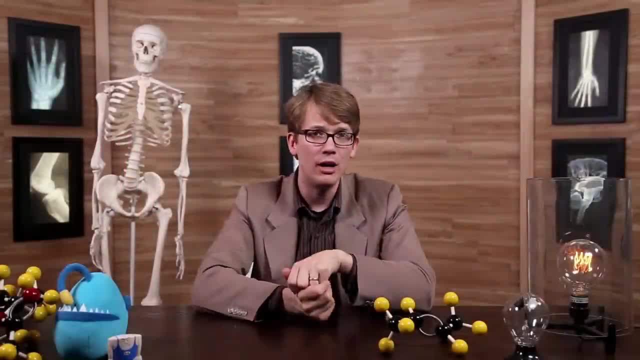 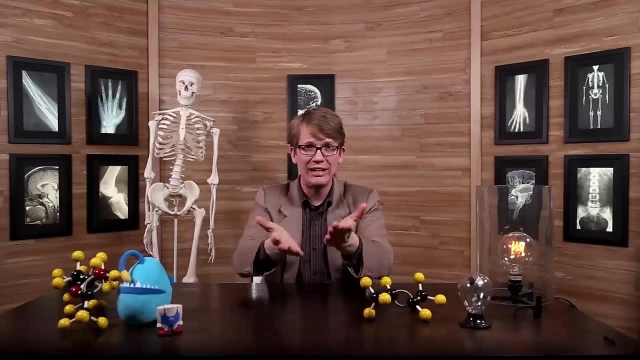 Essentially it's like a verbal map, So over time, anatomy has developed its own standardized set of directional terms that describe where one body part is in relation to another. Imagine a person standing in front of you. This is what is called the classic anatomical position, where the body is erect and facing. 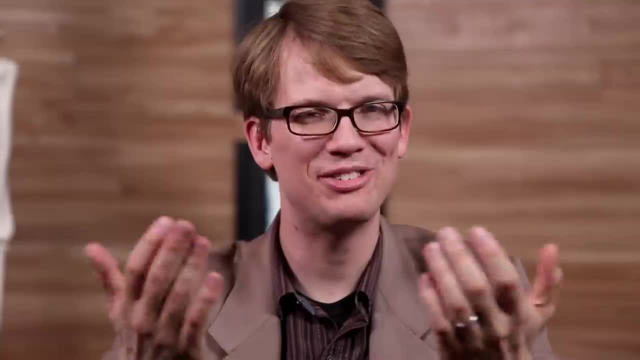 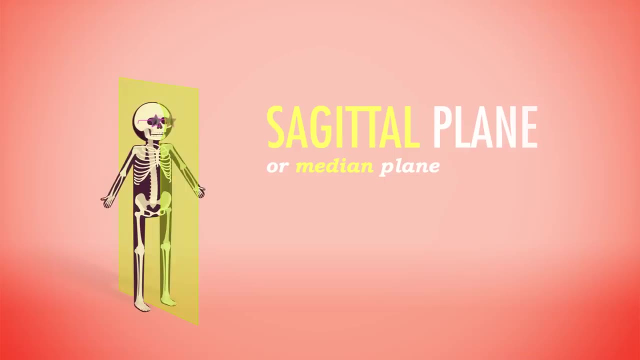 straight ahead with arms at the sides and palms forward. Now imagine slicing: Slicing that person into different sections or planes. Don't imagine it too graphically, though. The sagittal plane comes down vertically and divides a body or organ in left and right. 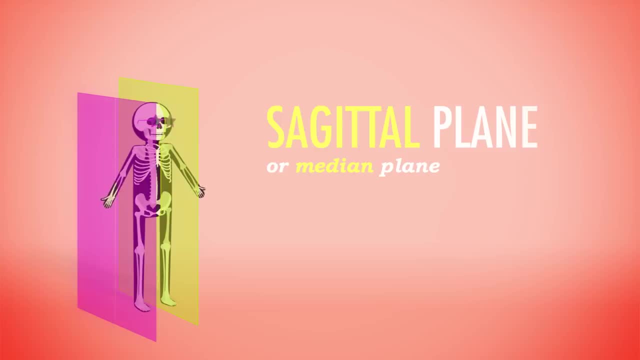 parts. If you imagine a plane parallel to the sagittal plane but off to one side, that plane is the parasagittal. The coronal or frontal plane splits everything vertically into front and back, And the transverse or horizontal plane divides the body top and bottom. 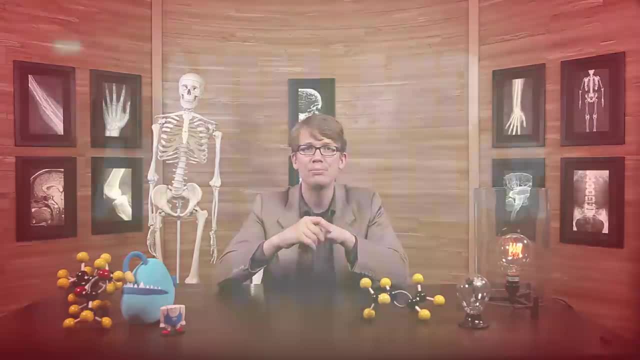 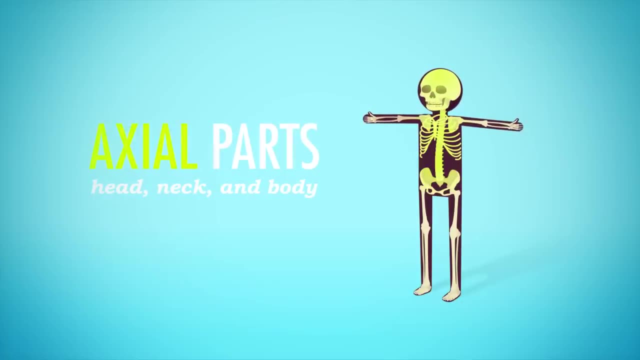 Look at that body again and you'll notice even more divisions, like the difference between the axial and appendicular parts. Everything in line with the center of the body- the head, neck and trunk- are considered axial parts, while the arms and legs, or appendages, are the appendicular parts that attach to. 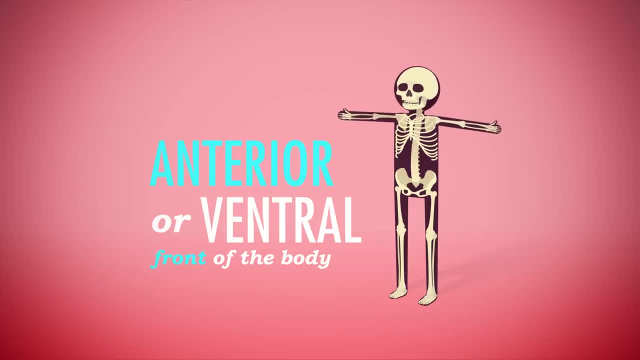 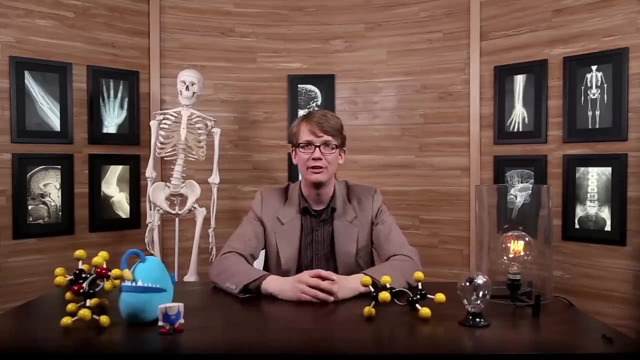 the body's axis. Everything in the front of your body is considered anterior or ventral, and everything in the back is posterior or dorsal. So your eyes are anterior and your butt is posterior, But you'd also say that your breastbone is anterior to or in front of the spine and 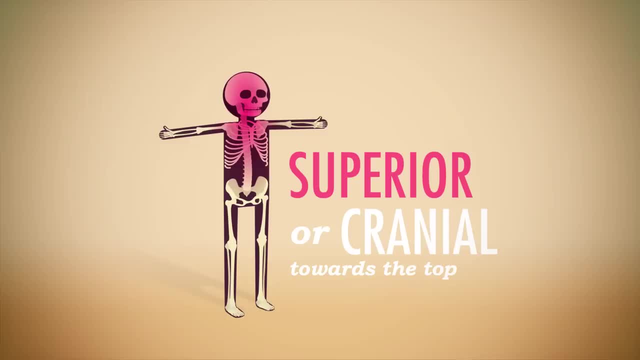 the heart is posterior to or behind the breastbone. Features toward the top of your body, like your head, are considered superior or cranial, while structures that are lower down are inferior or caudal. So the jaw is superior to the lungs because it's above them, while the pelvis is inferior. 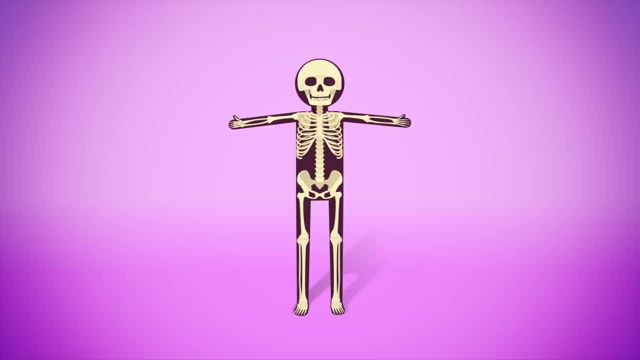 to the stomach because it's below it. And there's more. If you imagine a center line running down the axis of a body, structures toward that midline are called medial, while those farther away from the midline are lateral. So the arms are lateral to the heart. 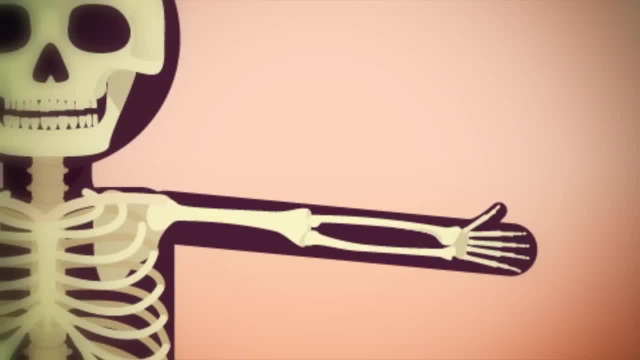 And the heart is medial to the arms. Looking at the limbs, your appendicular parts of your body, you'd call the areas closer to the center of the trunk proximal and those farther away distal. In anatomy talk, your knee is proximal to your ankle because it's closer to the axial. 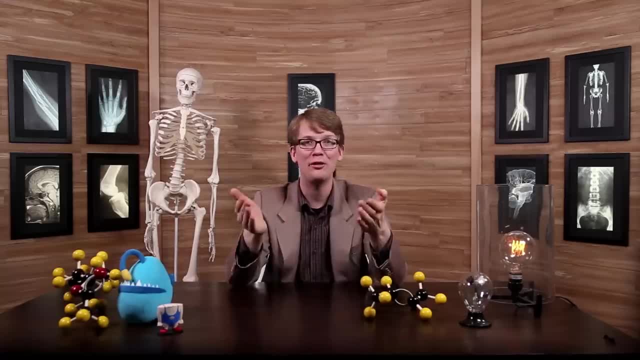 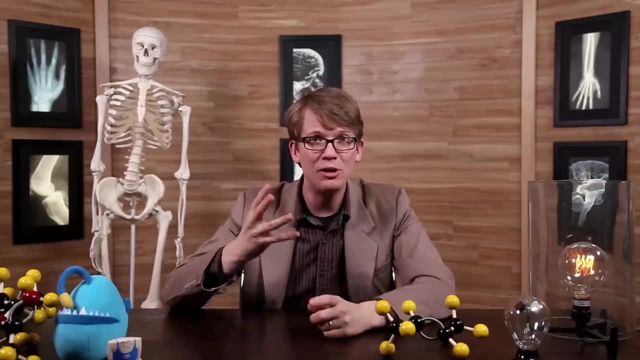 line, while a wrist is distal to the elbow because it's farther from the center. Okay, some pop quiz. I'm eating a club sandwich. I'm not. I wish I was, But imagine I am. I'm so ravenous and distracted that I forget to take out the little frilly toothpick at.